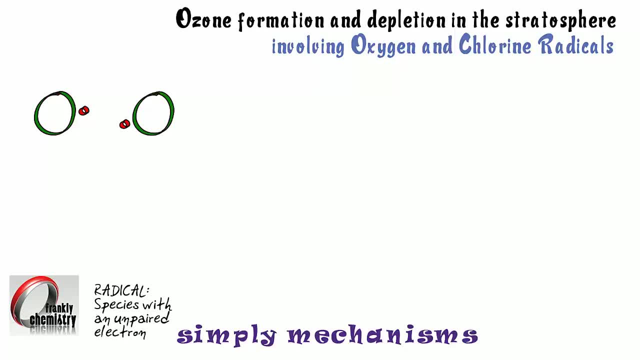 At the bottom. there you can see the radicals. You can see a radical is defined as a species with a non-paired electron. It's also known as homolytic fission. When the molecules split, both atoms were treated equally. We can summarize it more simply by taking the O2 molecule and show it being split into two oxygen radicals. 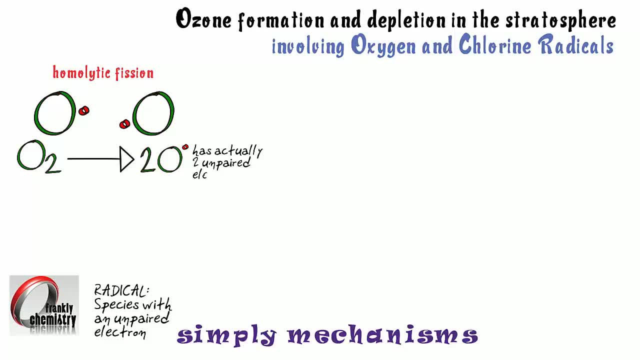 This is often how it's shown. However, I'd like to demonstrate that, in fact, oxygen radicals have not one, but two unpaired electrons. So let's look at this in better detail. at the top here, That's my oxygen molecule. then 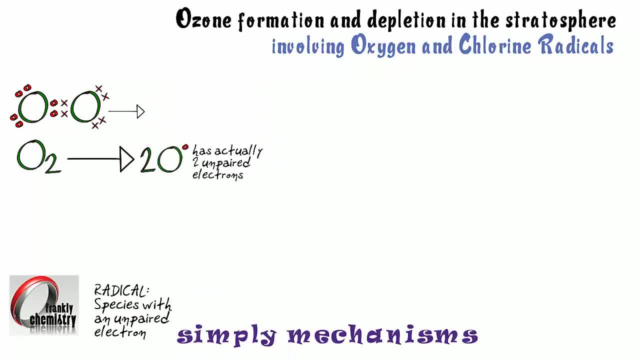 You can see, in the middle between the two oxygen atoms they are sharing two pairs of electrons. When the oxygen molecule splits, this is essentially what's happening. We're ending up with two oxygen atoms with six valence electrons Up at the top. here we'll build up the electronic configuration. 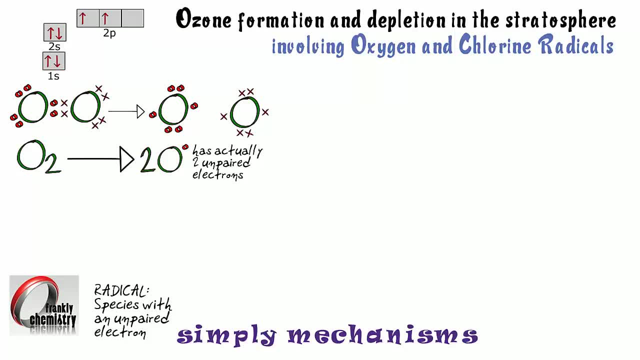 Let's see where these eight electrons go: Two into the 1s level and the other six go into the second energy level. If you look at 2s and 2p, you'll see there that we have two lone pairs and two unpaired electrons. 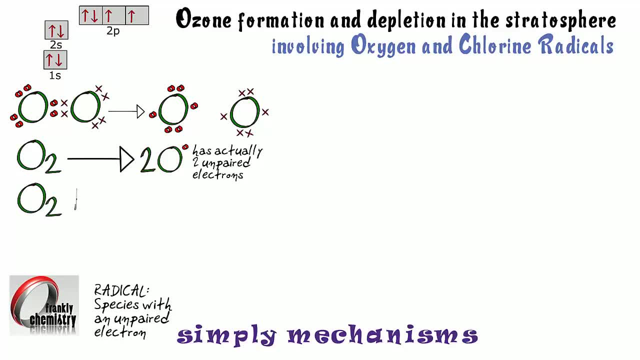 So the oxygen atom, or oxygen radical, actually has two unpaired electrons. You can show it either with one dot or, better still, with two dots to represent the two unpaired electrons. This is how ozone is formed in the solar system. It's formed in the stratosphere. 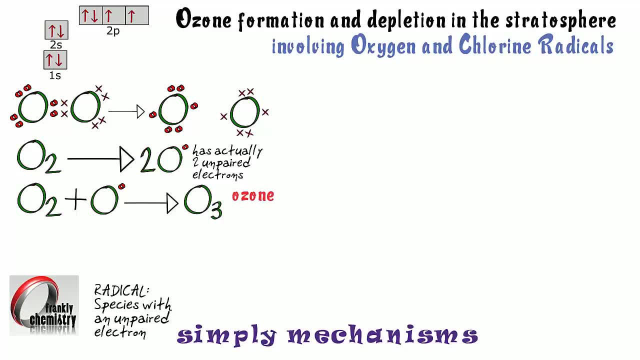 An oxygen molecule will hit one of those radicals and that forms our ozone molecule, And ozone shields us against the damaging UVB radiation which causes skin cancer, amongst other things. At the bottom here I'd like to show you how the electrons are assigned in the ozone molecule. 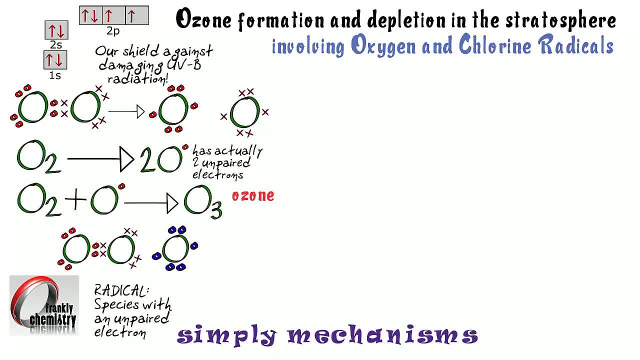 So I'm bringing in my oxygen molecule together with my oxygen radical and reassigning the electrons there. Here we go In that ozone molecule. you can probably make out there, with the electrons being shared, that we have a double bond between the middle oxygen and the one to the left. 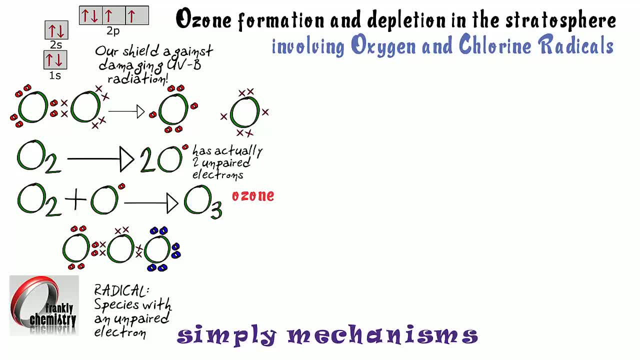 and a single bond between the oxygen and the one to the right. Now I've put a minus value, minus sign on that oxygen to the right because it effectively has seven electrons. It's got its six blue spheres, which represent its six original electrons, But it's also gained a share in that pair of electrons represented by the two crosses. 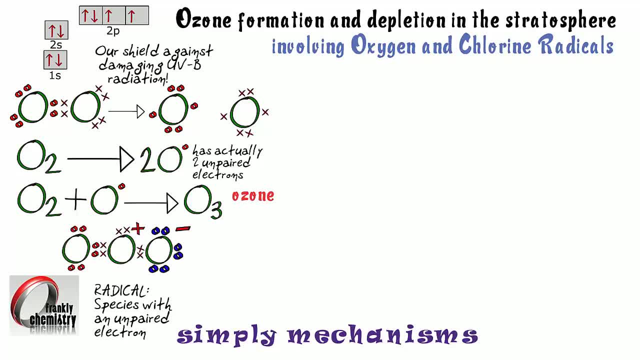 A share in a pair means you're up an electron And therefore it has a negative charge. Meanwhile the oxygen in the middle, if we count the number of electrons it has, it's got one lone pair, plus it has the share in three pairs. 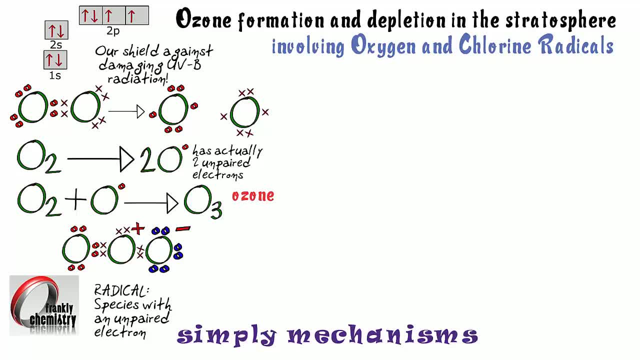 A share in three pairs adds up to three, So three and two is five. It's down an electron effectively, and that's why it's shown with a positive charge. So that's been my look at ozone formation. Now let's look at ozone depletion. 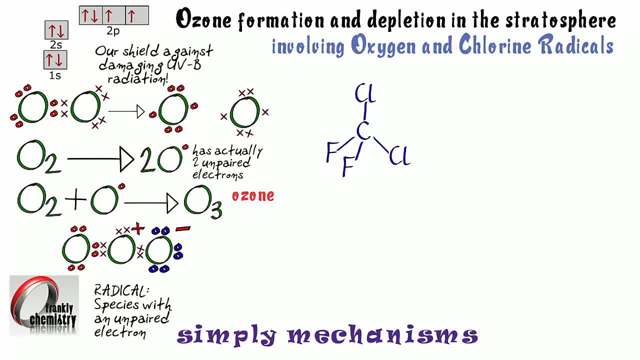 Caused in particular by molecules like this, called CFCs- chlorofluorocarbons. This particular one is dichlorodifluoromethane. These enter the stratosphere about ten miles high up from their usage on Earth. 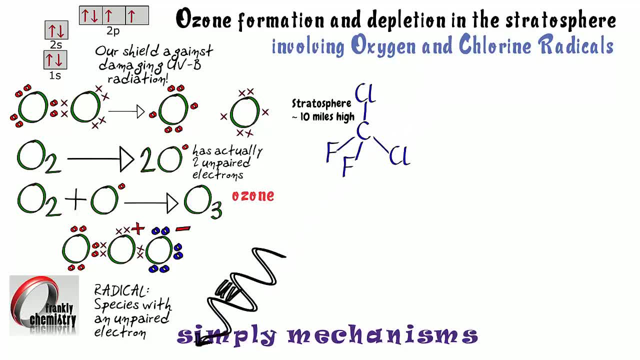 In the past they would have been used as propellants in aerosols and as refrigerants in fridges. You see our UV rays coming through here again And, as they did with the oxygen molecule originally there at the top left, they have a tendency to break the CCL bond. 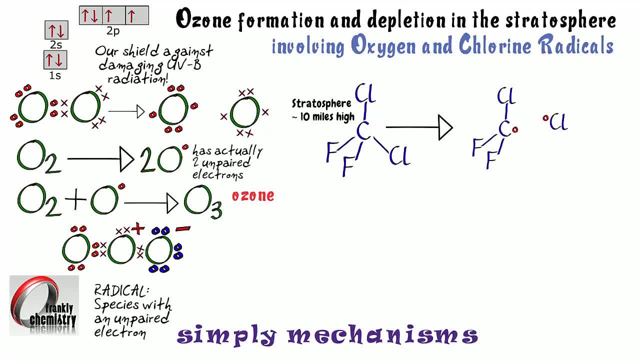 They happen to have an energy that comes into resonance with the vibration of the CCL bond, causing some of these molecules to split as you see there, producing two radicals And in particular that chlorine radical. So let me bring over an ozone molecule, now, O3,. 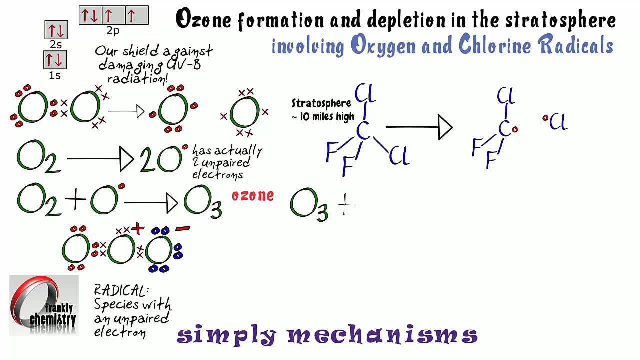 and see how that chlorine radical begins a cycle of destruction. There's my chlorine radical Again. a radical is a species. A radical is a species with a non-powered electron. And let's see what it does: It collides with the ozone molecule. 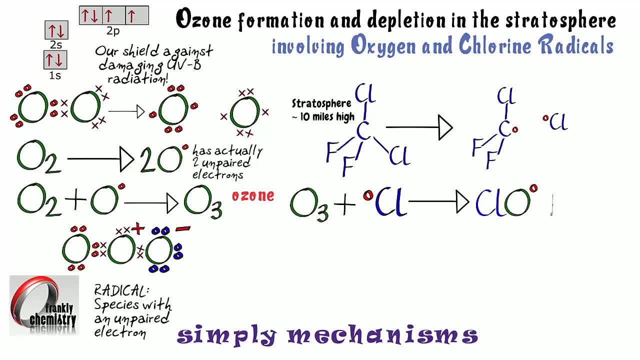 and causes the ozone molecule to split to produce a molecule of oxygen- O2, together with this radical CLO. And let's see what the CLO radical does next. The important thing is that that step has broken down one molecule of ozone into oxygen.